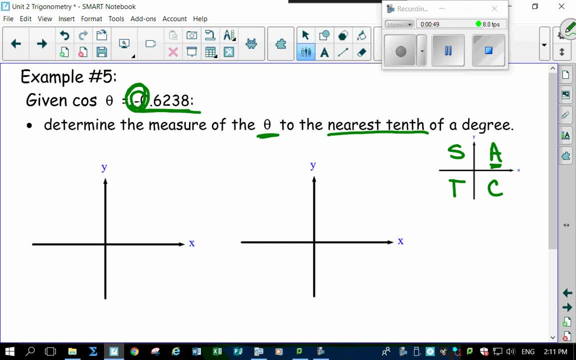 negative. Well, cosine is positive because everything's positive here. Cosine is positive here, meaning you got an angle out here and you have an angle out here. Okay, so let's do the first one. There's the angle out here. We're gonna find the reference angle, of course, to the x-axis, So we're gonna draw. 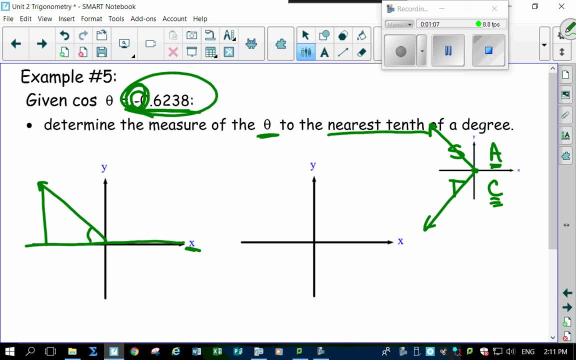 a triangle out here. We're gonna note that the cosine of this angle is- well, let's clean it up, because I can't even read that anymore- is negative 0.6238.. We're also know that it's going to be down in this direction, So I'm gonna put 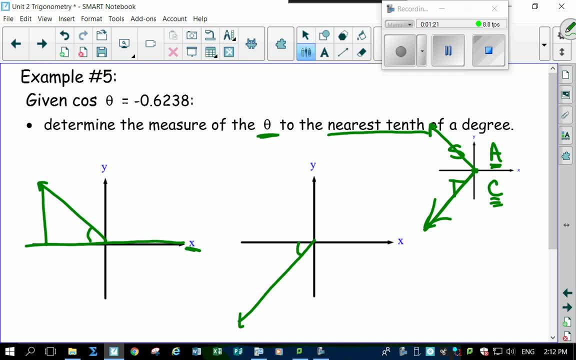 it down here. and again, there's my reference angle. Okay, there's my nice 90 degree triangle, because, again, reference angle is to the x-axis. So how do we do this? Well, real simple: Don't include the negative. Why? Because the negative tells me it's here and it's here. Once you're dealt with that, you 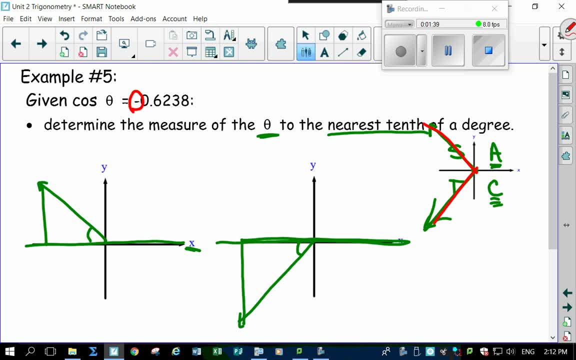 don't need that negative anymore. It's done, It's history. You know the angles are going to be here and here because of the cast rule. You're done. Just use the point six, two, three, eight. Well, let's find out what theta then is. How do we do? 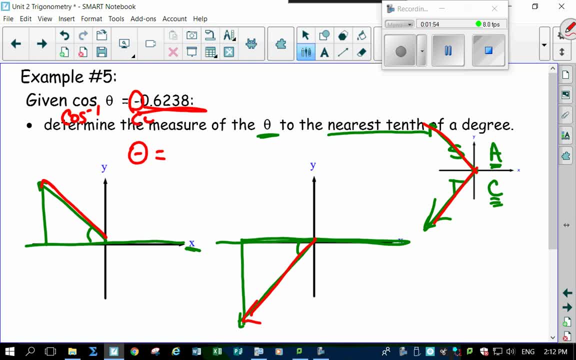 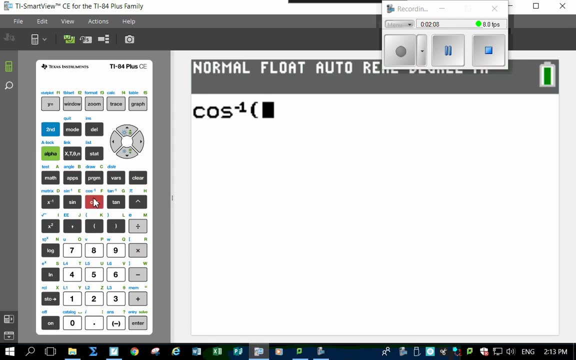 that Well remember from math 10c. you take the inverse of both sides, So the inverse of the cos of both sides cancels us out, leaving us with a theta equals two, So the inverse cos of 0.6238.. Put up our calculator: Inverse cos of 0.6238.. 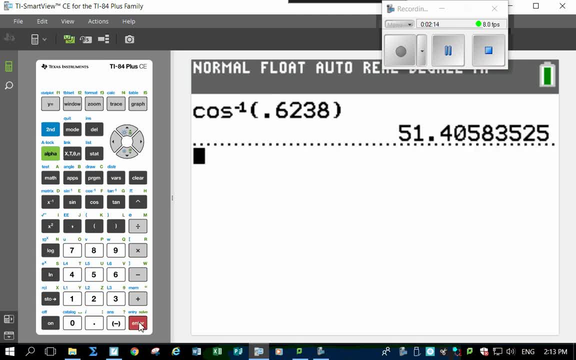 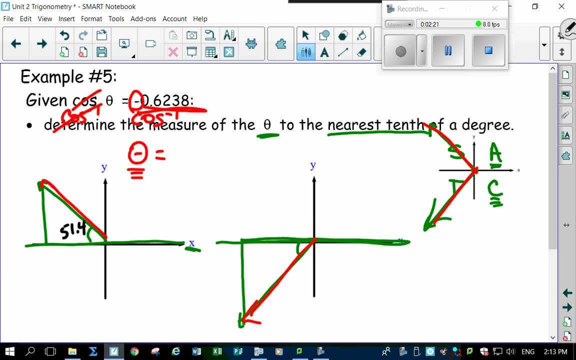 Boom Enters. That works out to be fifty one point four degrees. Okay, that means my reference angle is fifty one point four. That one and that one, Okay, and it's going to be fifty one point four. Now, remember, don't use the negative, because 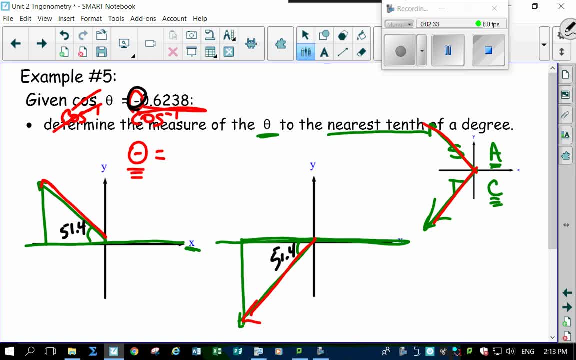 the negative will might just throw those numbers off for you. Now, how do we solve this now? What is our angle in standard position? Remember, standard position starts here. it goes all the way over to here, All right. so doesn't that look like it's not what? quite 180.. As a matter of fact, it's 180 subtract 51.4 and you're.